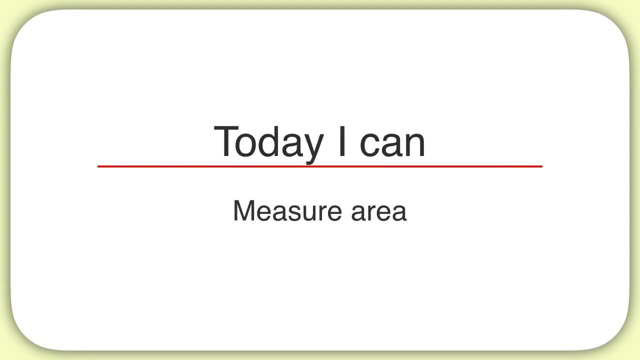 Today we are learning how to measure area. When I measure something like this piece of string, I might measure its length. I could measure that it has a length of 3 units, But what about something like this square? Well, when I'm measuring the size of something, 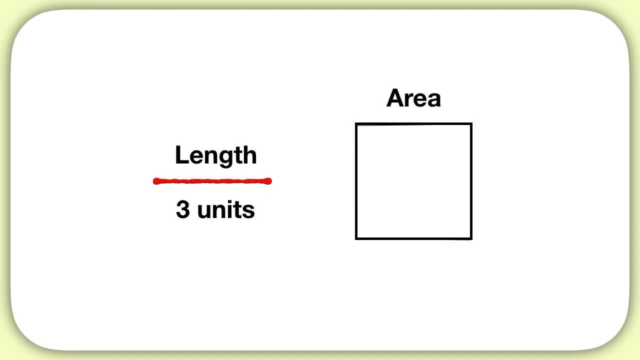 like a square. I do it by using area. How do I do that? Well, if we take a look at this square, we could think about covering it with smaller squares of a set size. We call these small squares one-unit square. Now we can see how many of these unit squares fit inside. 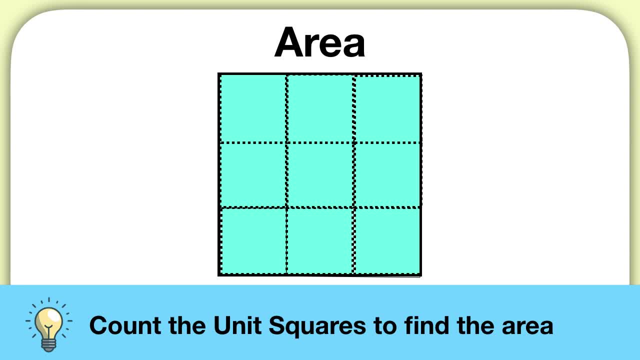 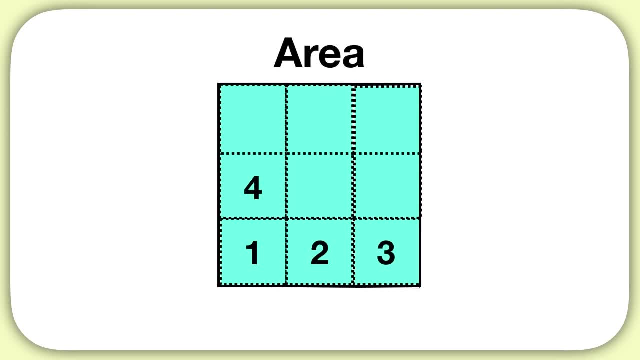 of our big shape, Then all we need to do is count up the unit squares to find the area For this shape. we could count: it takes 1,, 2,, 3,, 4,, 5,, 6,, 7,, 8,, 9 unit squares to fill. 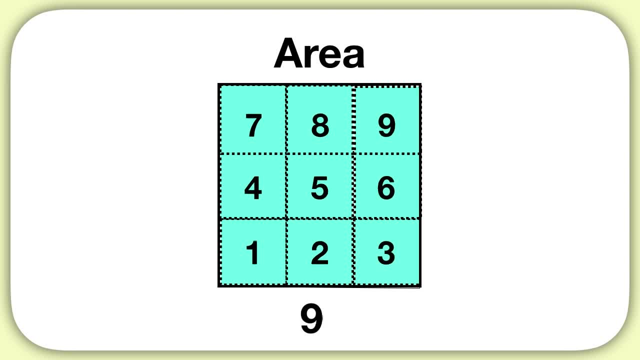 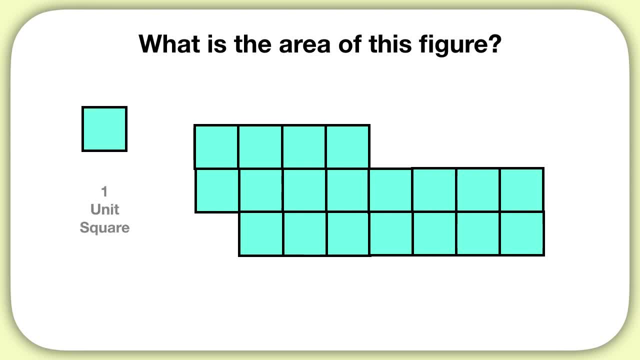 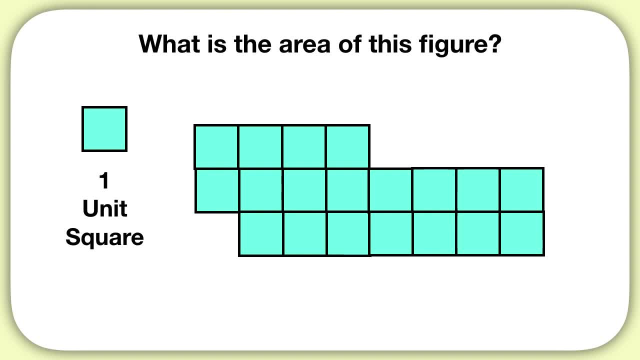 this shape. To find the area of a shape, just count the number of unit squares inside of it. How many unit squares are in this shape? Well, we could count all of the unit squares in this shape. If you did this, you would find that it has an area of 20 square units. 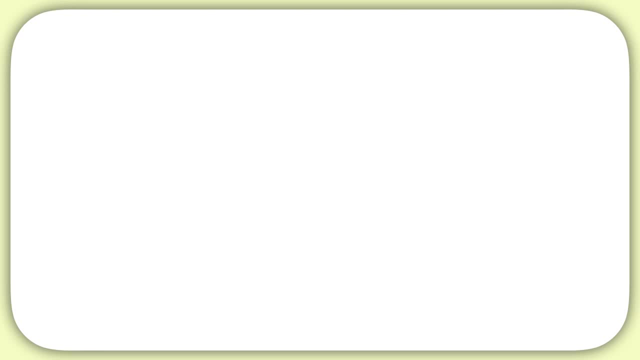 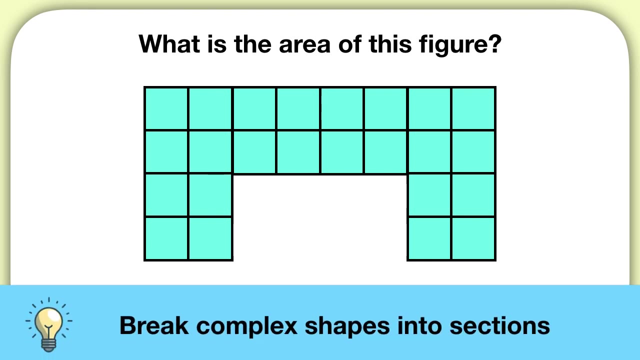 Well, here's another problem to practice with. What is the area of this figure? Well, my advice, when you're dealing with a complex shape like this, is to break it into sections so it's easier to count. We could first focus on this green section right here. How many?